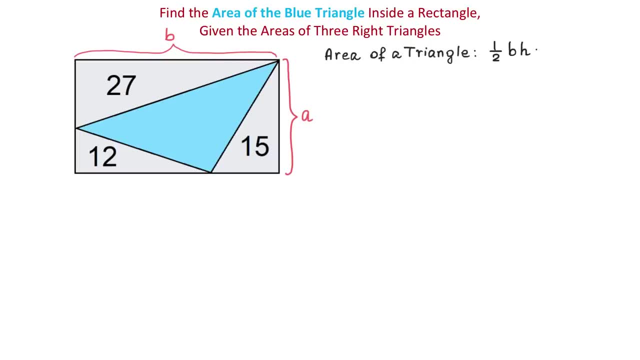 1 half by the base and by the height In this triangle, we can say that the base is B and let this height be X. Then we can write that 1 half times B and times X equals 27.. Now let's take a look at the triangle, whose area is 15 square units. 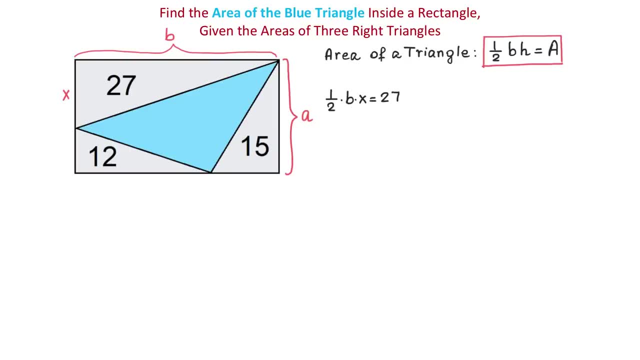 In this triangle. we can say that the height is A and let's call the base Y. Then we can write that 1 half times Y and times A equals 15.. Now what about the base and the height of this triangle If this side of the rectangle is B and this part is Y? 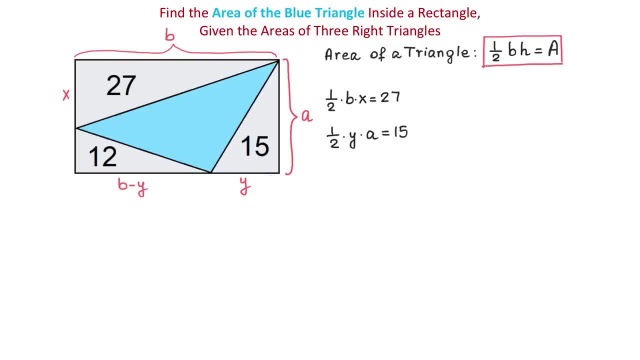 then this part will be B minus Y. And if this side of the rectangle is A and this part is X, then this part will be A minus X. Then we can write that 1 half multiplied by B minus Y and multiplied by A minus X equals. 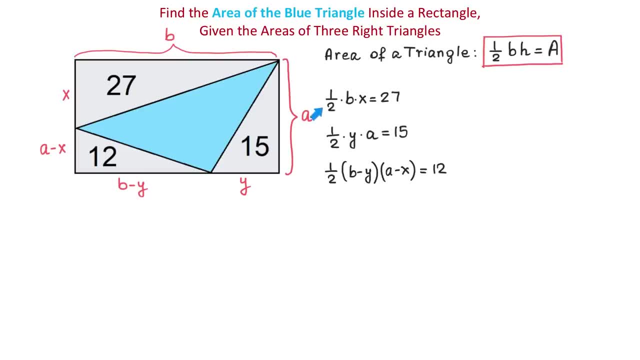 12.. So so far we have these equations that represent the areas of these triangles, but as you see, they have a lot of variables, so we will try to use substitution to eliminate some of these variables. First we will solve this equation for X and in the first step we will multiply both sides. 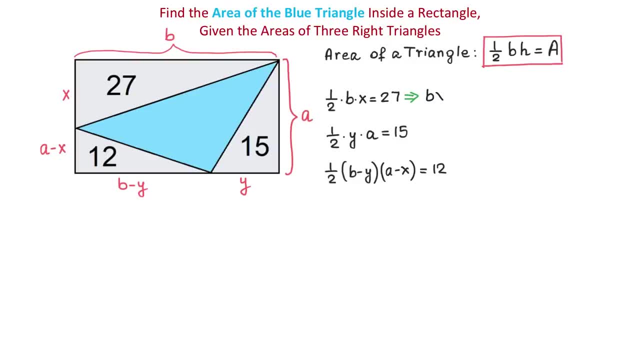 by 2. Then we will have BX equals 54. And now, if we divide both sides by B, we will get that X equals 54 over A over b. Now the next equation will be solved for y, and we will start by multiplying both sides by 2.. 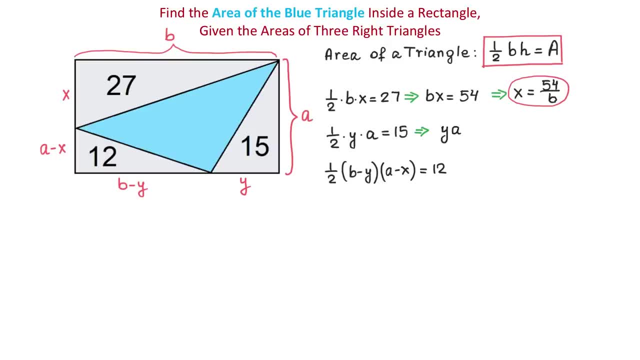 Then we will get that y times a equals 30. Then if we divide both sides by a, y equals 30 over a. Now in the third equation we will replace y with 30 over a and x with 54 over b. 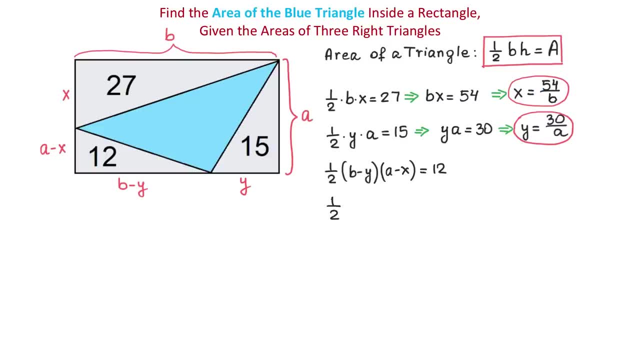 Then we will have 1 half times b minus 30 over a times a minus 54 over b equals 12.. Now, as you see, this equation has only two variables, and these are a and b. Now let's simplify this equation and let's see if we can solve it. 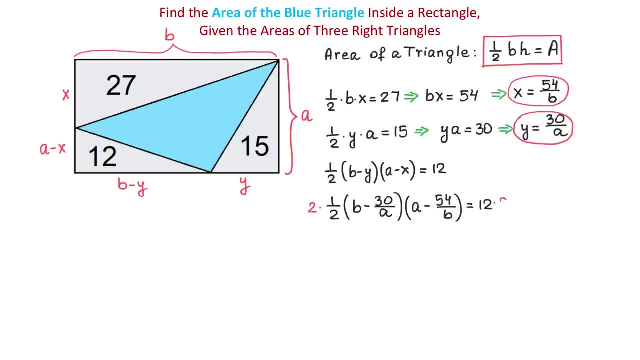 First we will multiply both sides by 2.. Then on the left side, 2 and 2 will cancel. Then we will remove the parentheses by using FOIL. So b times a is ab, Then b times negative 54 over b will be b. 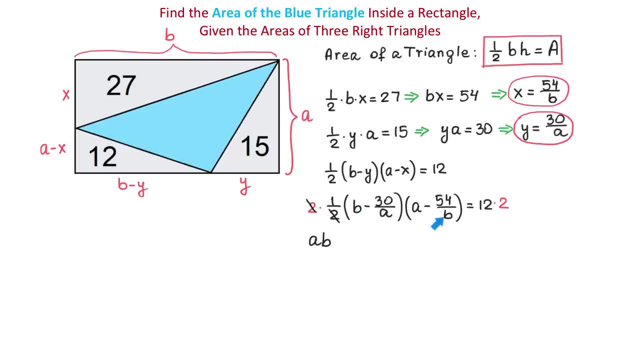 Then b times a will be negative 54 because b and b will cancel. Then negative 30 over a times a is negative 30 because a and a will cancel. So we will write minus 30. Then negative 30 over a times negative 54 over b will be positive 1620 over ab. 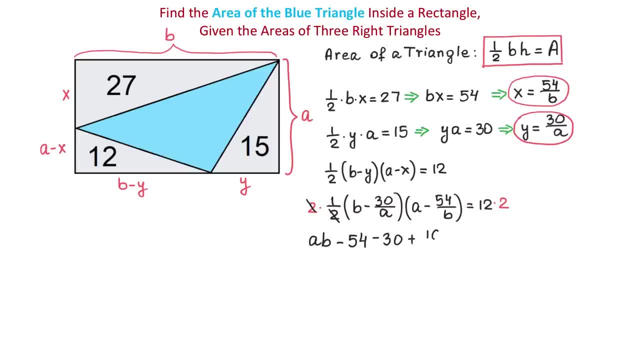 So we will write plus positive 1620 over a times a, minus 1620 over ab. Then on the right side we will have level 24.. Now we will subtract 24 on both sides and we will have ab minus 54, minus 30 and then minus 24 plus 1620 over a times a, be 0. 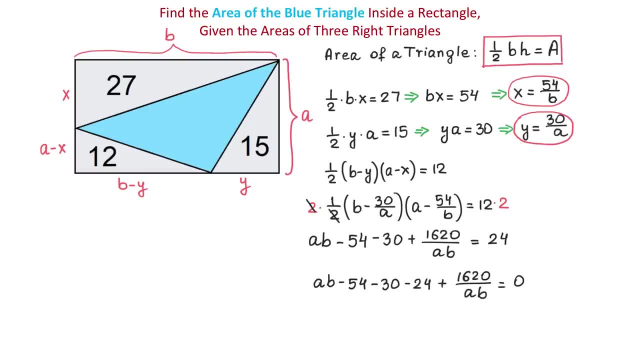 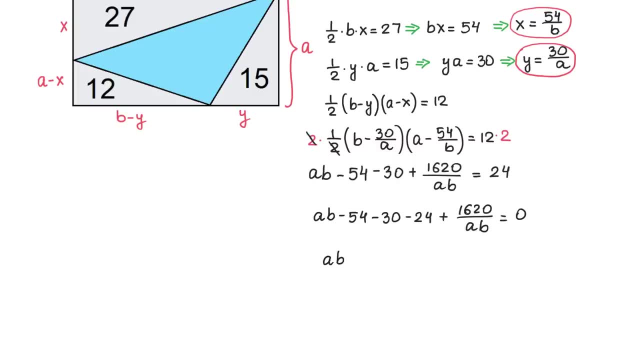 So we will write: minus 30, minus ab, minus 1620 over a times b equals 0. Then if we combine these three numbers together we will get negative 108, then we will have AB minus 108 plus 1620 over AB equals zero. 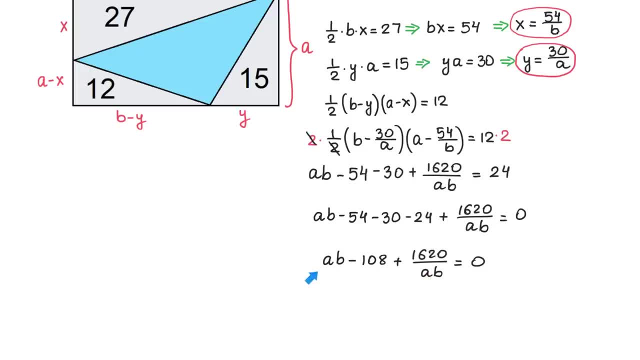 Now to get rid of this denominator. we will multiply both sides of this equation by AB. On the left side we will use the distributive property. Then AB times AB is AB squared AB times negative. 108 is minus 108 AB and AB times 1620 over. 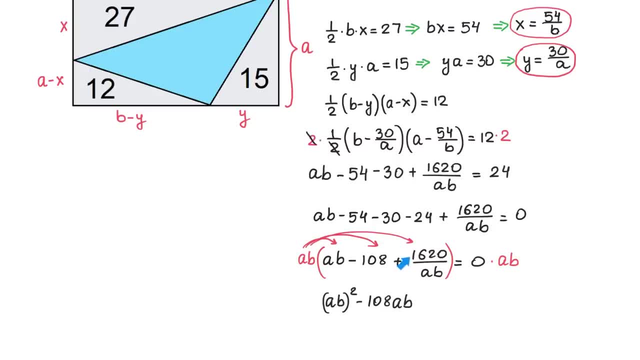 AB will be 1620 because AB and AB will cancel, So we will have plus 1620 over AB, And on the right side we will have zero. Now let's recall that a quadratic equation has the form: AX squared plus BX plus C equals. 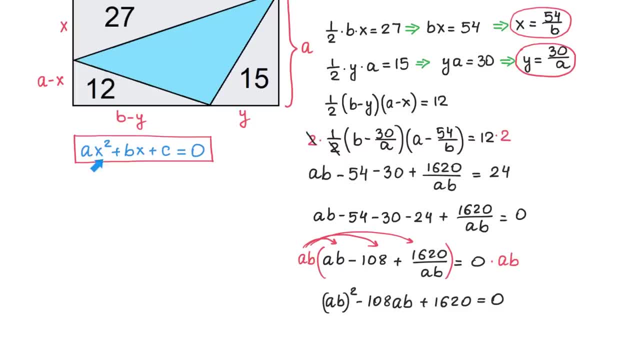 zero. In this equation, the variable is X, and A, B and C represent numbers. Now do you see that the equation we got here is also a quadratic equation. So we have A, B and C equal to zero. Now let's recall that a quadratic equation has the form A, B and C equal to zero. 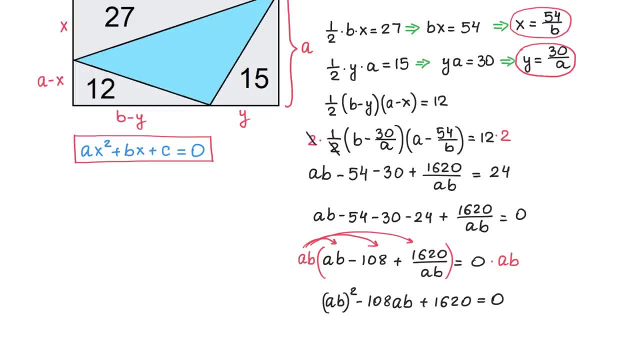 Now do you see that the equation we got here is also a quadratic equation. Now do you see that the equation we got here is also a quadratic equation Where the unknown is the product AB. If we can solve this equation, we can find the product AB. 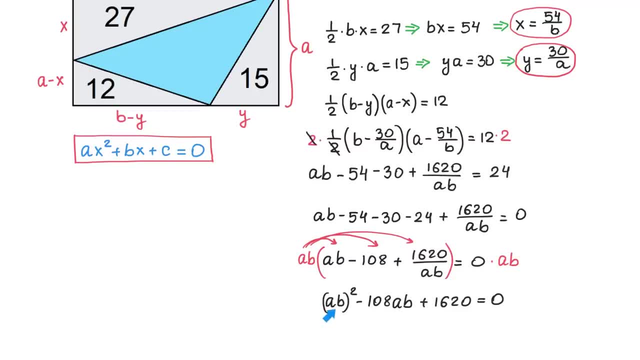 And the good part is that this product, AB, represents the area of the rectangle. To solve a quadratic equation, we can use factoring if it's possible, or we can use the quadratic formula. For the equation to the left, the quadratic formula is X. 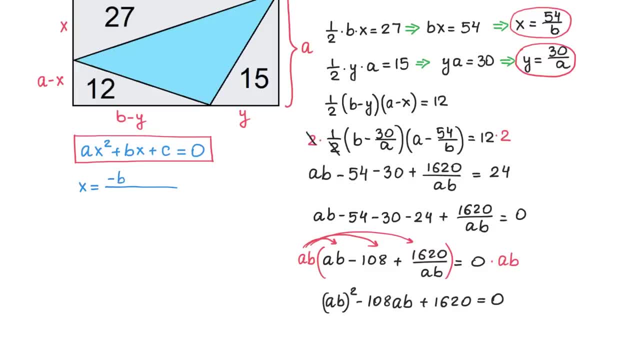 X equals fraction negative B, plus or minus square root of B. squared minus 4AC, all over 2 times A. If we use this formula for our equation, then we will get the following: The unknown AB equals fraction bar. and now, in place of negative B, we need the opposite.